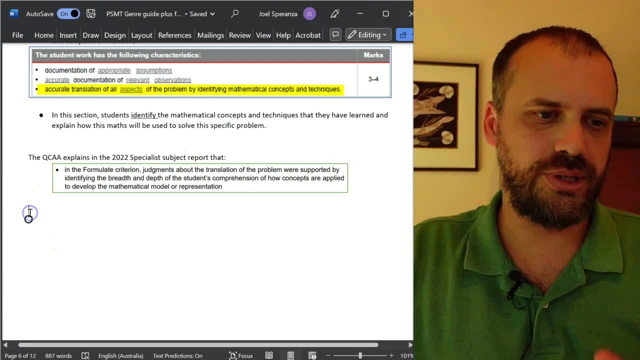 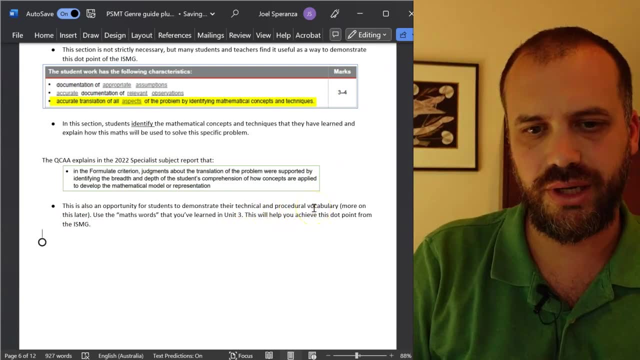 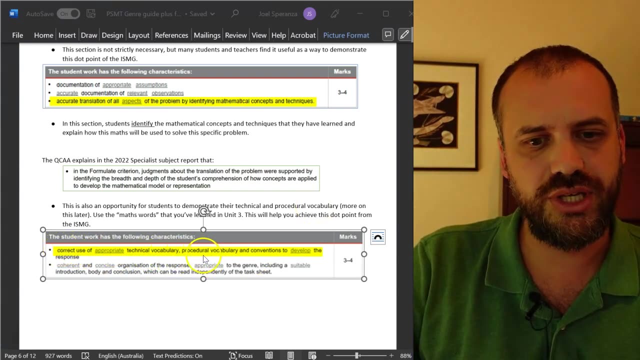 to do that. There's another reason I really like this section: because I think it's a golden opportunity for you to demonstrate your technical and procedural vocabulary. Of course you want to do that because that's part of the ISMG. That's how you'll be marked on your technical and procedural. 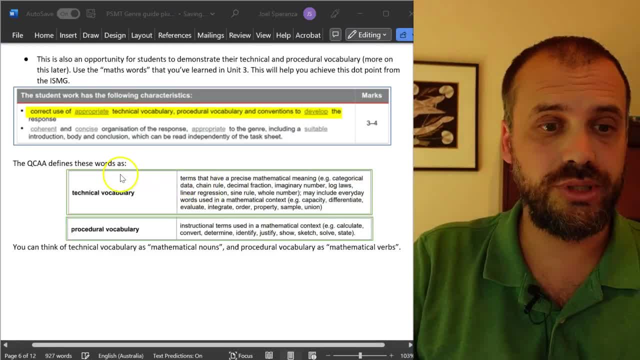 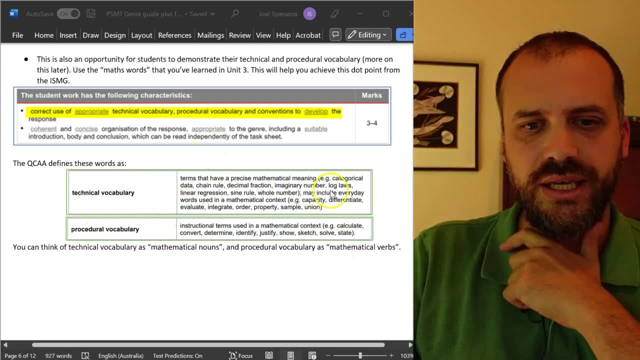 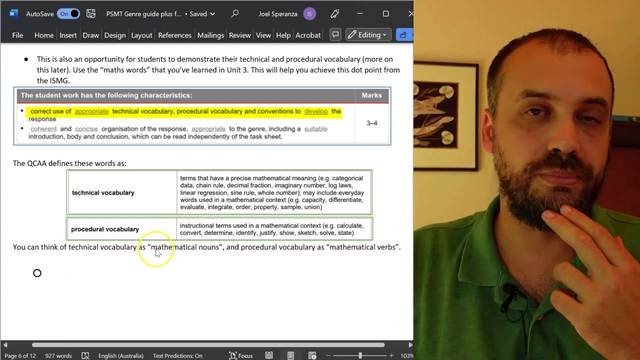 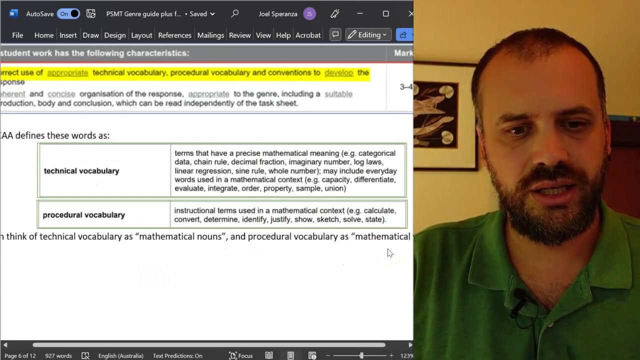 vocabulary. If you dive into the syllabus documents, you can find out different types of definitions for technical vocabulary and procedural vocabulary, And they give some examples there. I think of these things as technical vocabulary being mathematical nouns and procedural vocabulary being mathematical verbs, And if you take a look at their procedural 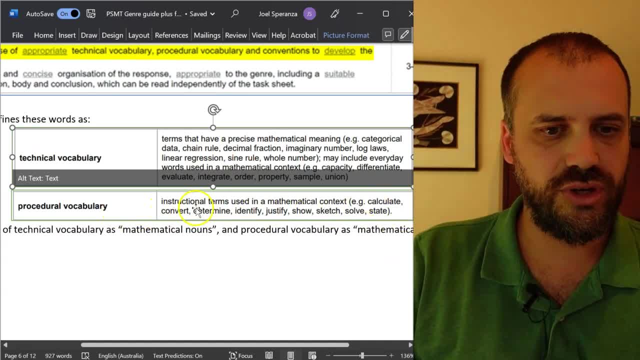 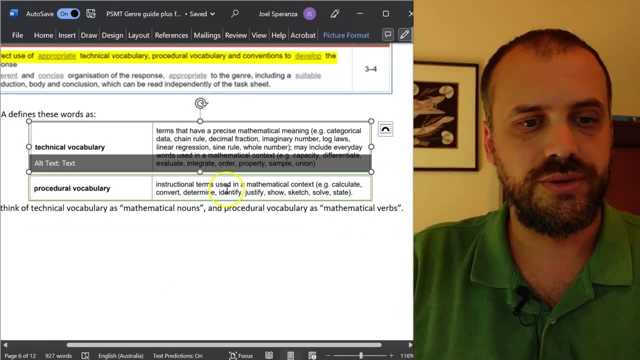 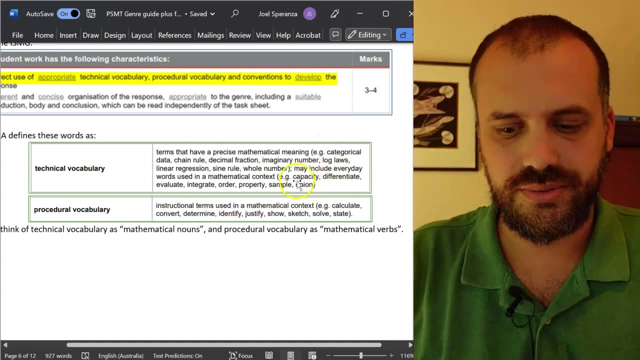 vocabulary: definition: calculate, convert, determine, identify, justify, show, sketch, solve, state. these are all verbs. They're all doing words. If you take a look at their technical vocabulary, it's all nouns, It's all things. 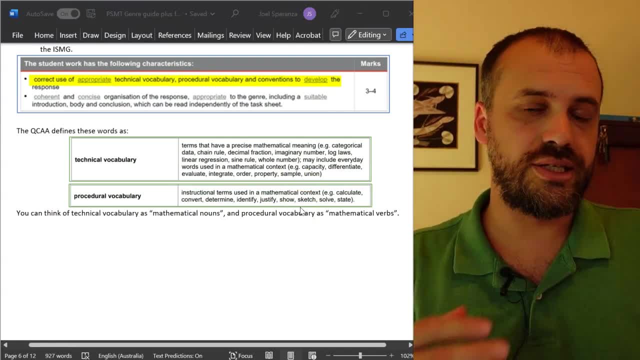 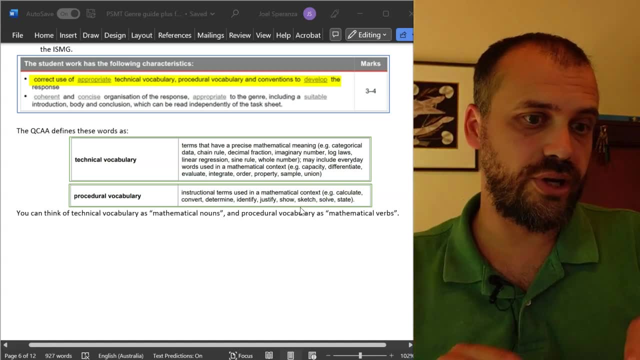 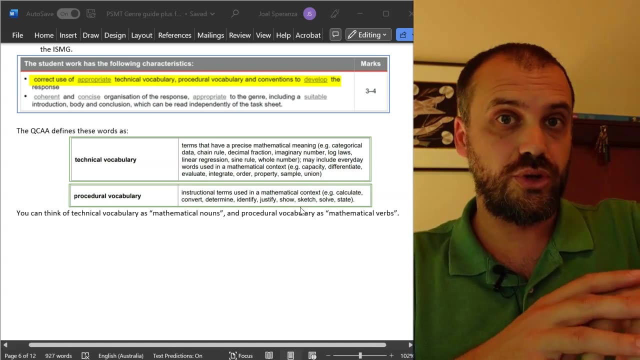 If you were to get together with a group of your friends and sit down with your textbook with the topics that you've been covering and look for technical vocabulary and procedural vocabulary and put it into your PSMT. so maybe you do a big brainstorm and you come up with 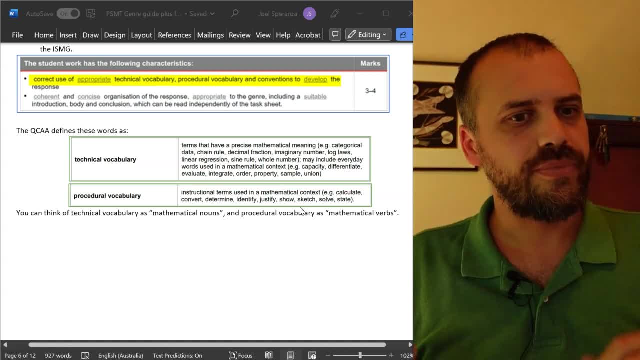 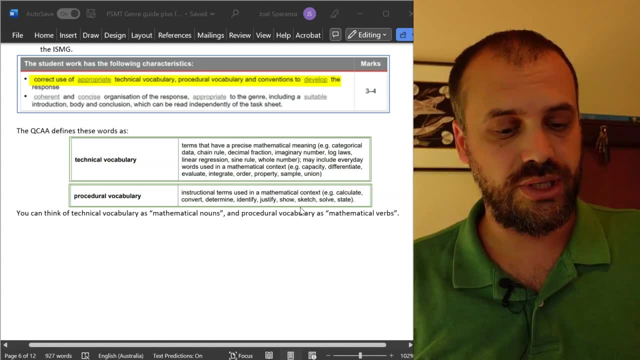 50 words And you go great. these are all going to be in my PSMT. Now you'll know if you've done a good job if, at the end of your PSMT, a friend of yours can hit control F. search for the. 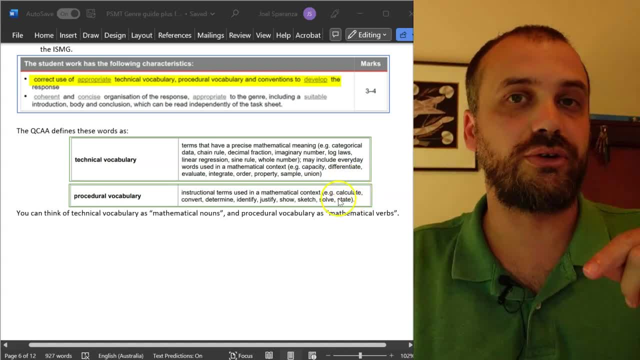 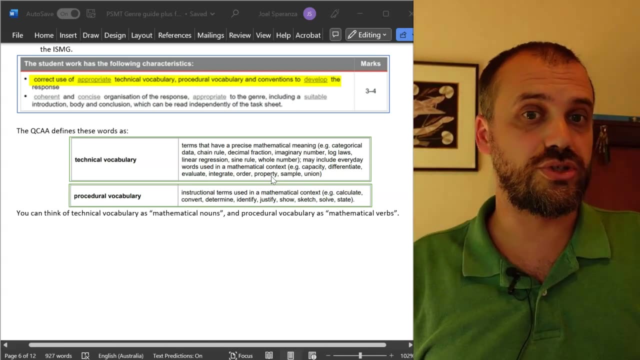 word calculate and it'll pop up. or calculated. perhaps Search for the word integrate or integration or whatever it might be, and it pops up somewhere. So, coming up with a list of words and then making sure that you're using those words in your assignment by using 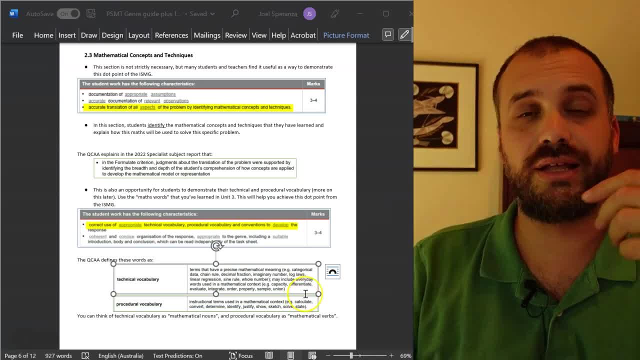 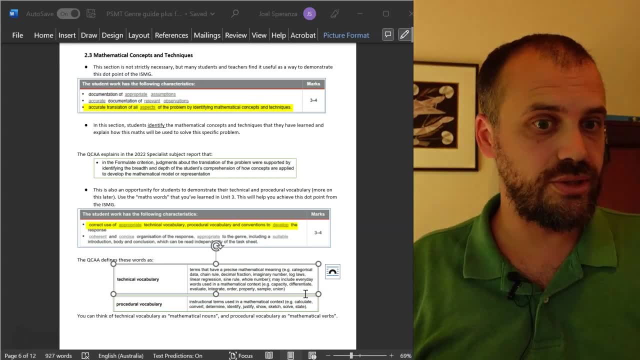 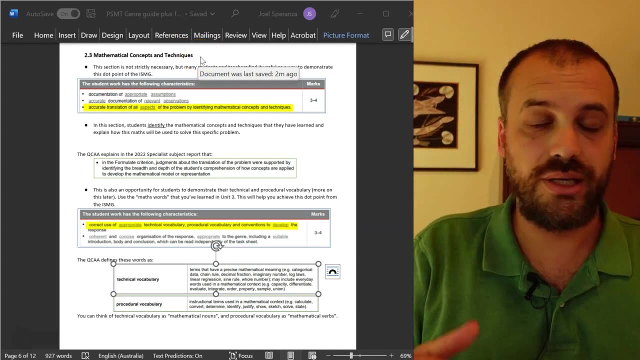 the old control F good idea. It's usually at this stage of the video when I say: and here's some examples of like fantastic student work. I'm not doing this this time because: one, because this section is sort of controversial, it's never really appeared in a subject report and also this dot point. 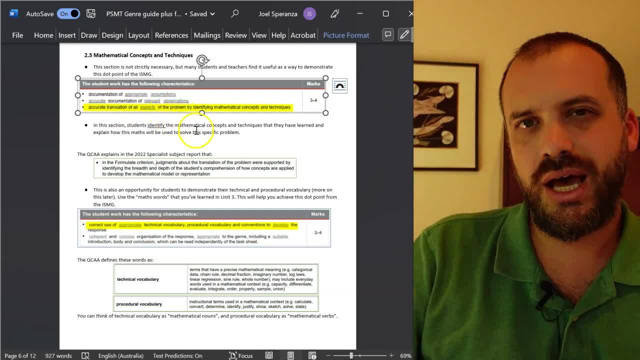 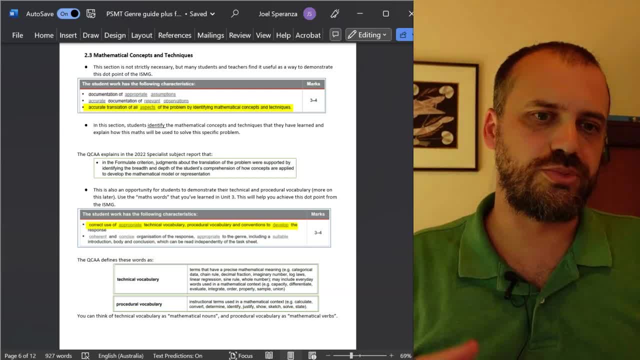 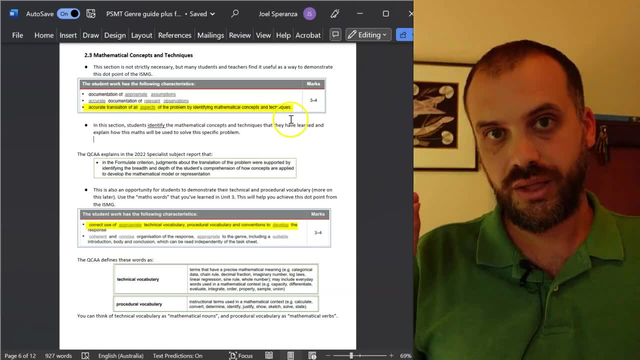 holistic approach to marking it. a teacher is supposed to look at the entire assignment and determine whether a student has done this or not. so controversial section. put it in there. don't put it in there. i've made my case, you decide. 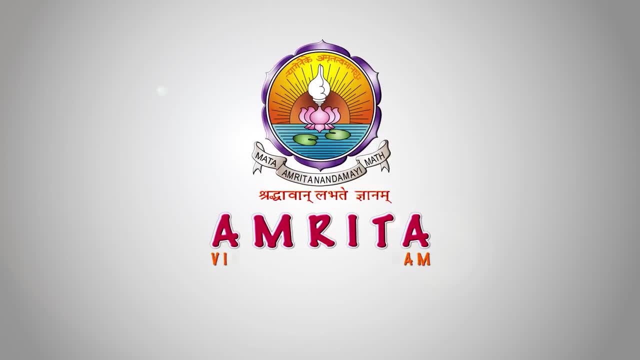 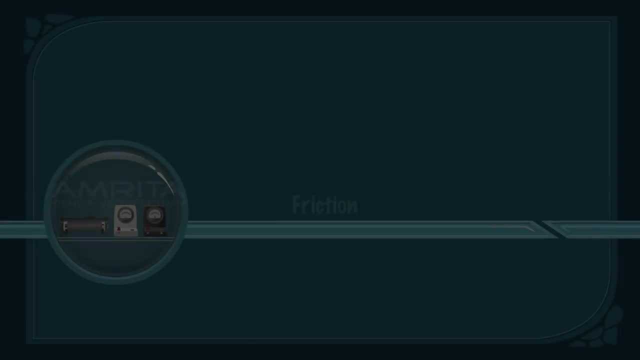 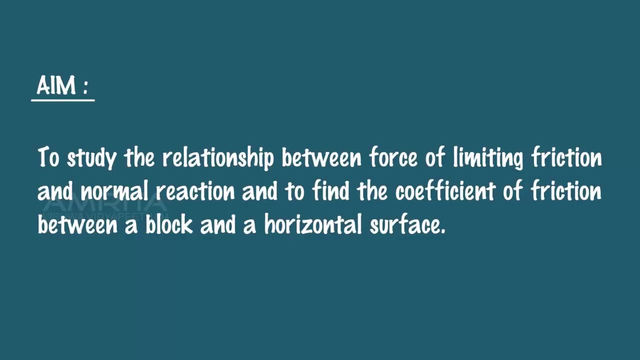 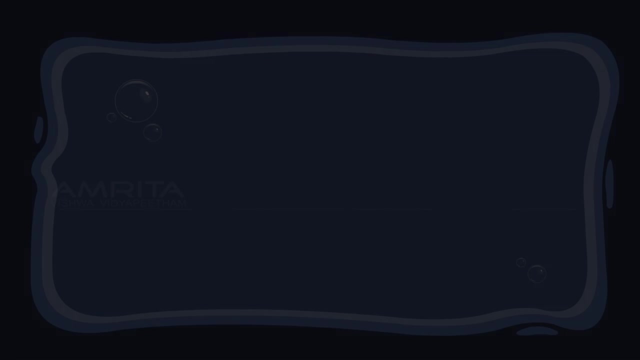 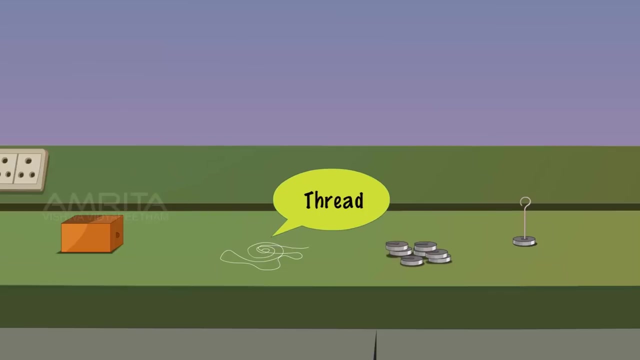 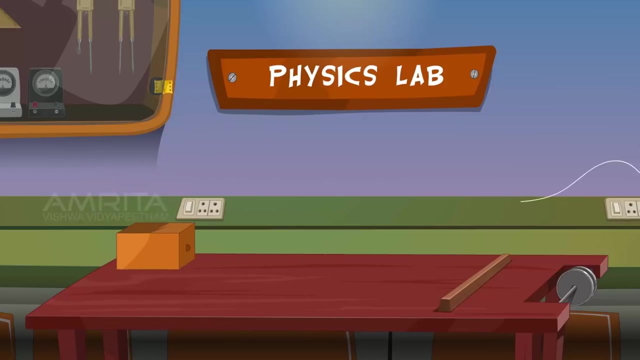 Friction. To study the relationship between force of limiting friction and normal reaction and to find the coefficient of friction between a block and a horizontal surface. Materials required: Wooden block, Thread, Slotted weights, Weight hanger. Take a wooden block with a hook on one end and place it on the table. 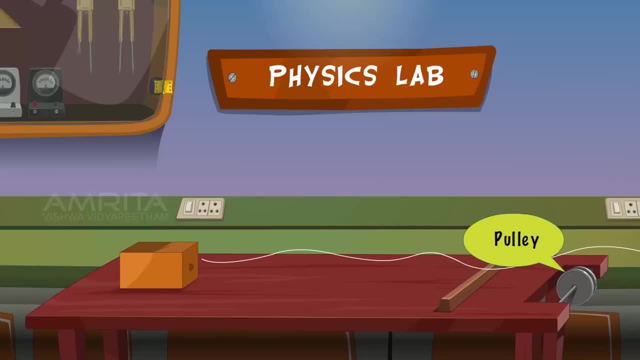 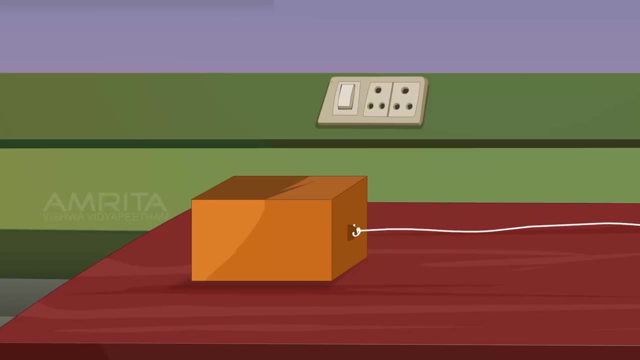 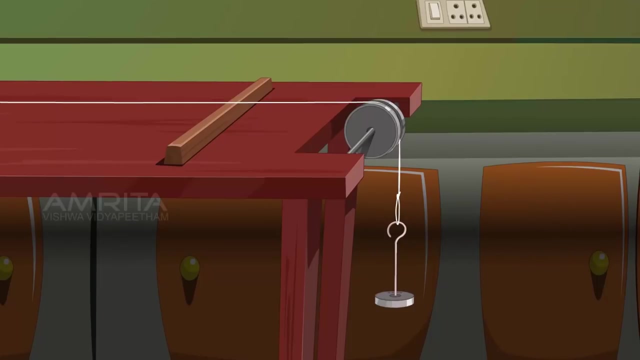 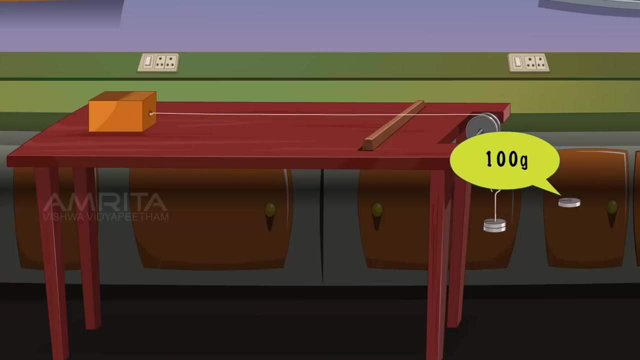 Take a piece of thread with a hook and tie the wooden block to it. Pass it over the pulley. Hang a 100g weight hanger on the free end of the thread and keep it vertical. Add 5 more 100g slotted weight to the weight hanger. 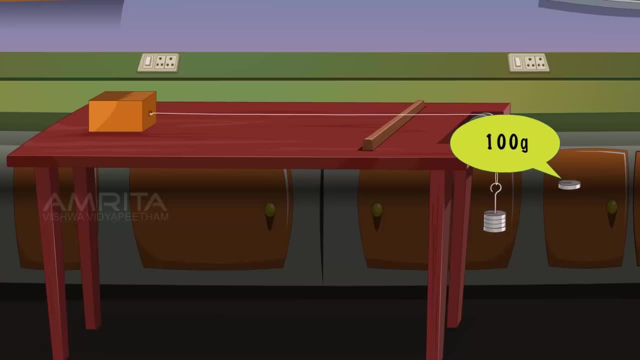